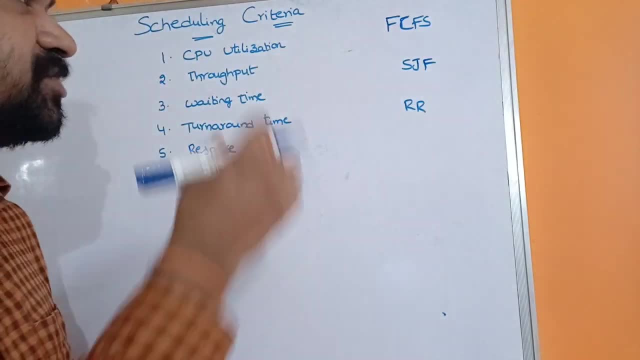 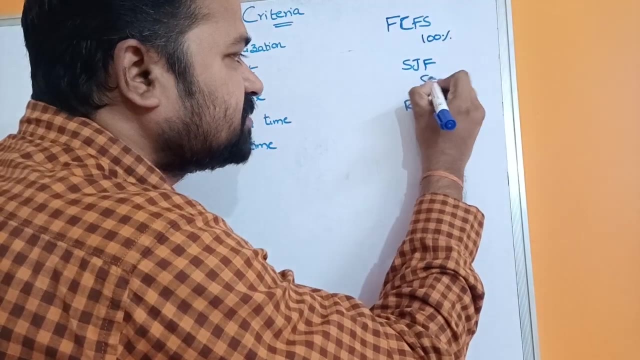 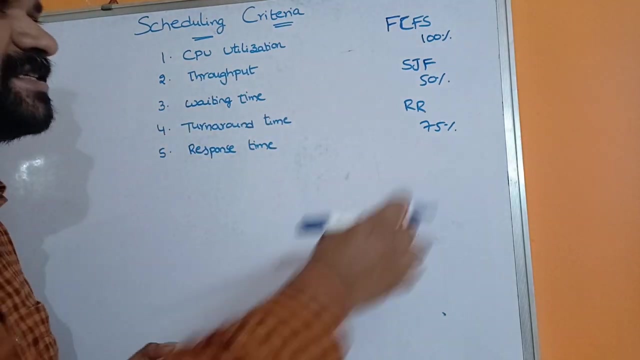 that algorithm is the best algorithm. Let us assume that FCFS algorithm CPU utilization is 100%, Whereas SAF algorithm CPU utilization is 50%, Whereas round robin scheduling algorithm utilization is 75%. Let us assume that these are the assumptions for CPU utilization. 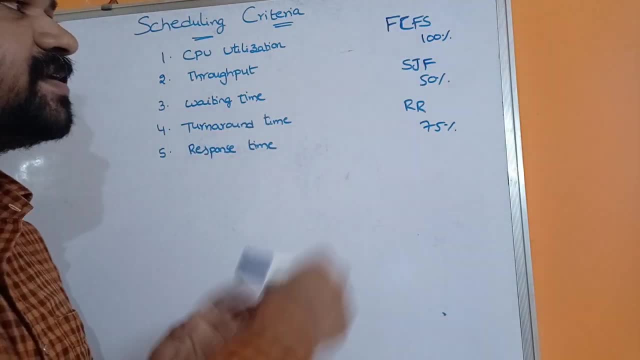 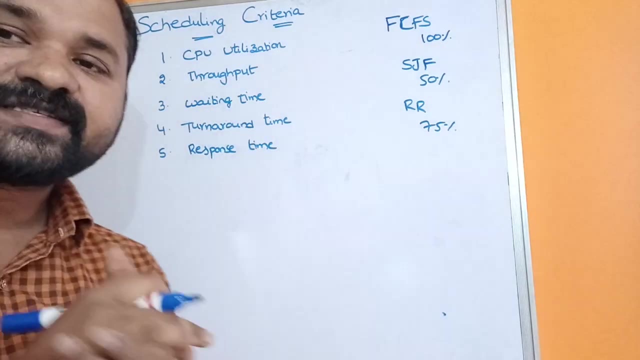 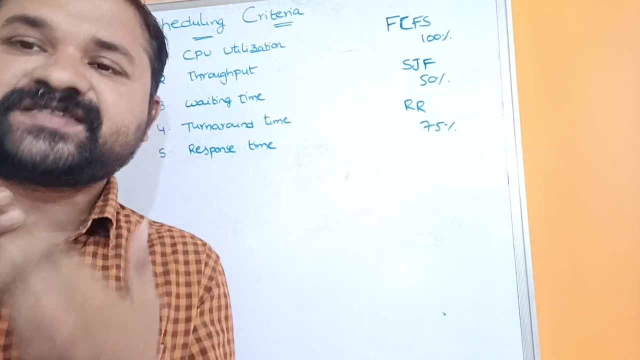 So out of all these, which is the bigger one? 100%. So we can say that FCFS is the best scheduling algorithm When considering CPU utilization. So here the point is, CPU utilization should be maximum So the system can make use of CPU in efficient manner. Then only we can. 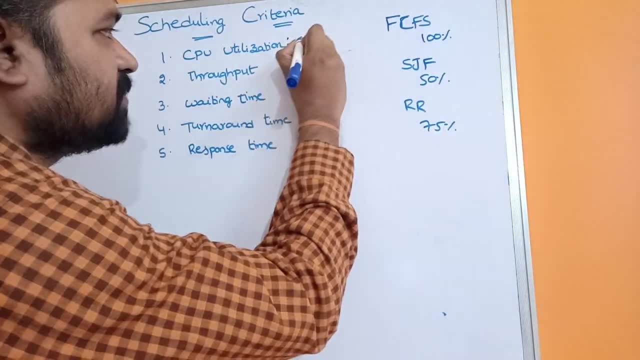 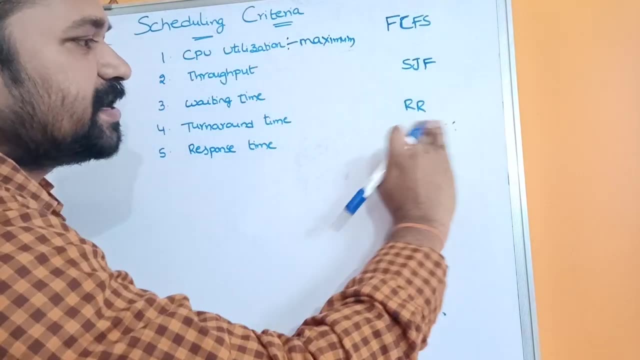 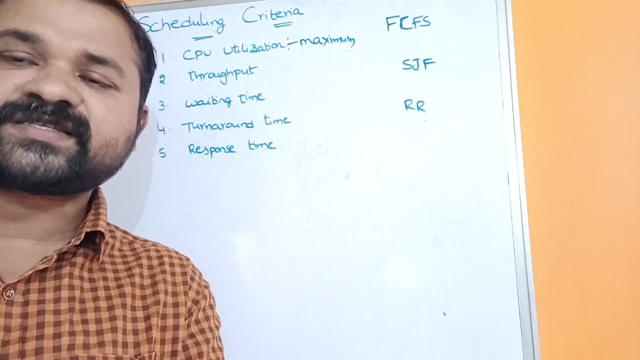 say that that is the best algorithm. So here CPU utilization should be maximum. So these are approximate values only. Okay, Now let us see the second factor. What is the second factor? Throughput. Throughput means how many number of processes are completed, their execution. 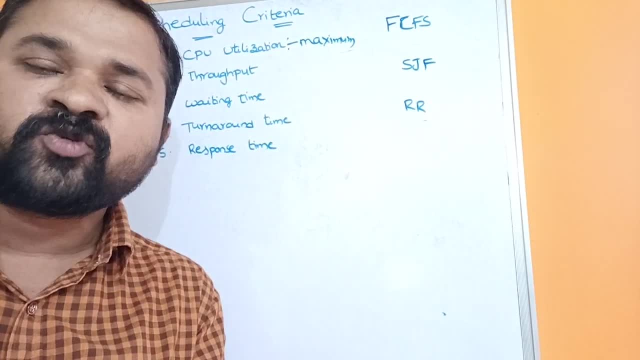 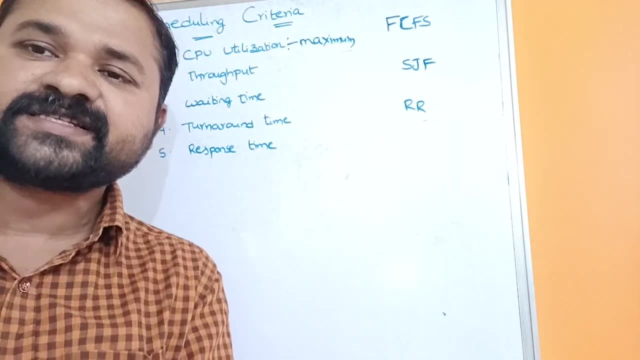 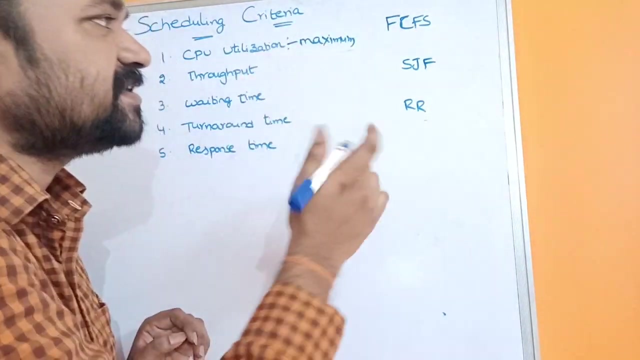 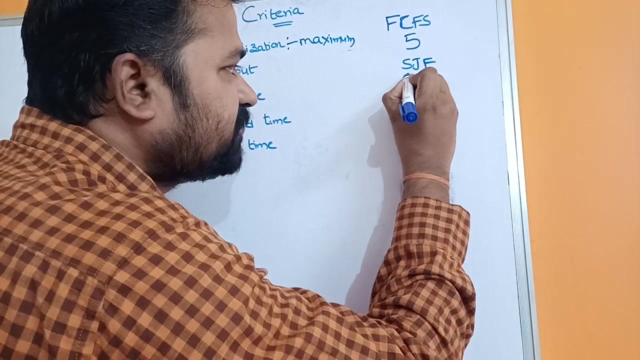 per a time unit. So how many number of processes we have completed per time unit? Here time unit may be 1 second or 10 seconds or 20 seconds or 1 minute or 20 minutes, Any time unit. Let us assume that in FCFS algorithm we have completed 5 processes execution in 1 second, Whereas in SAF we have completed 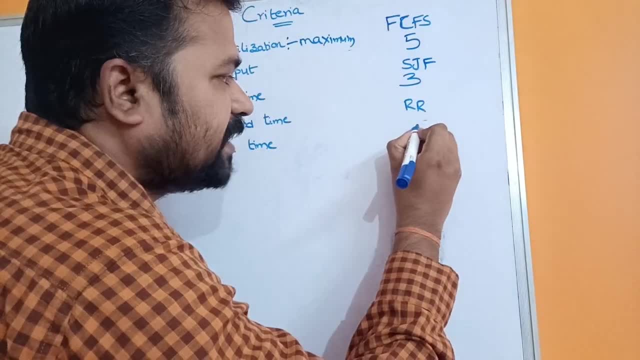 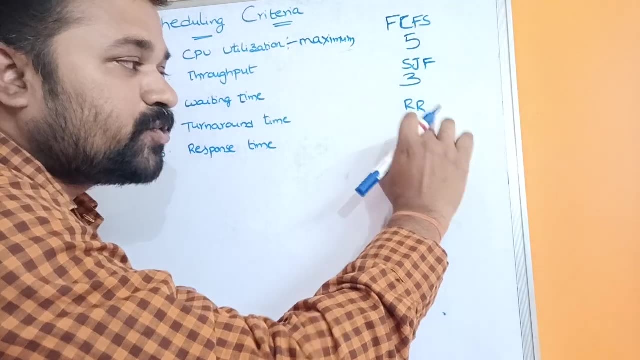 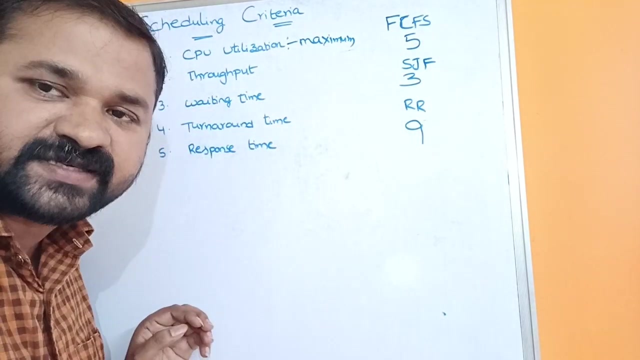 3 processes in 1 second, Whereas in round robin algorithm we have completed 9 processes in 1 second. So which is the best algorithm? now We can say that round robin is the best algorithm, Because by using round robin algorithm, we are executing more number of processes per a time. 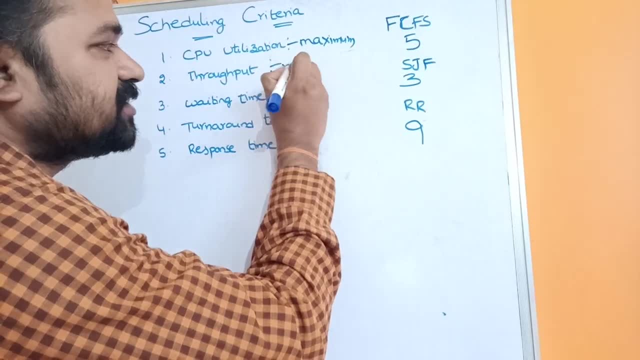 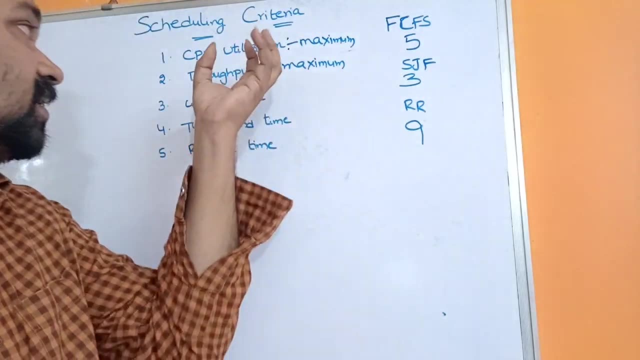 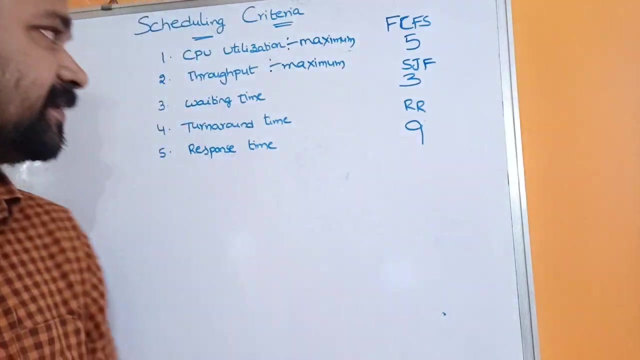 unit, So we can say that throughput is also maximum. So, as a user, our target is we have to utilize, we have to execute more number of processes per a second or per a time unit. Okay, Now let us see the second factor. So the second factor is waiting time. So what is waiting? 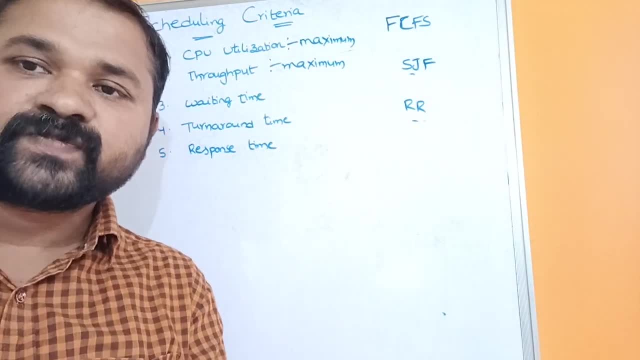 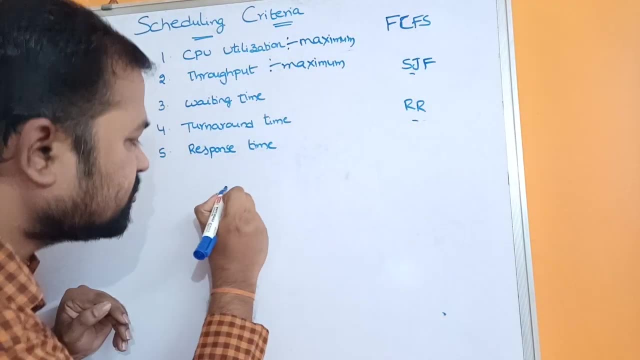 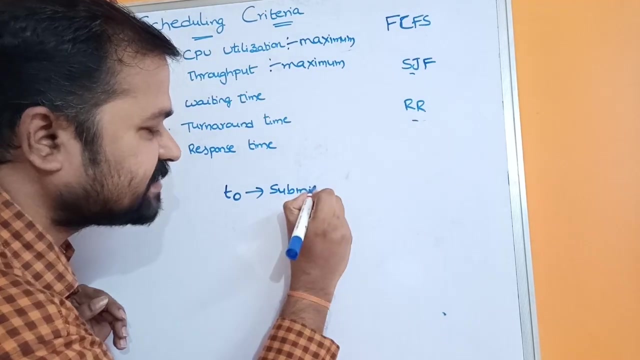 time. Waiting time specifies how much time a process waits in the ready queue for its execution. Let us assume that a process enters into the ready queue at t0,. a process is submitted. a process is submitted in the ready queue at a time t0. Whereas the process execution. 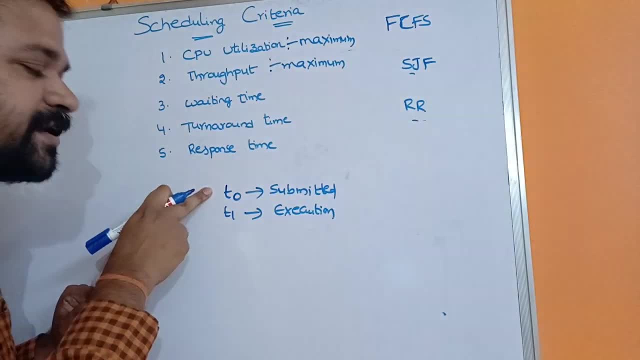 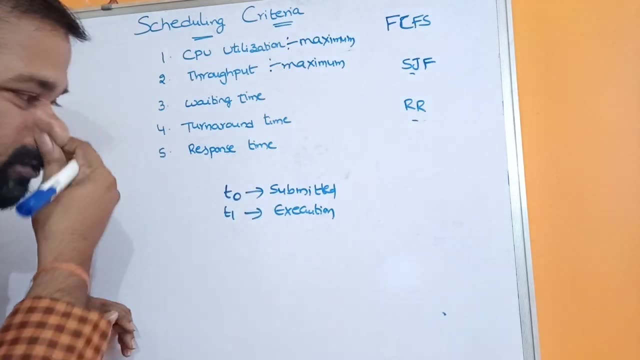 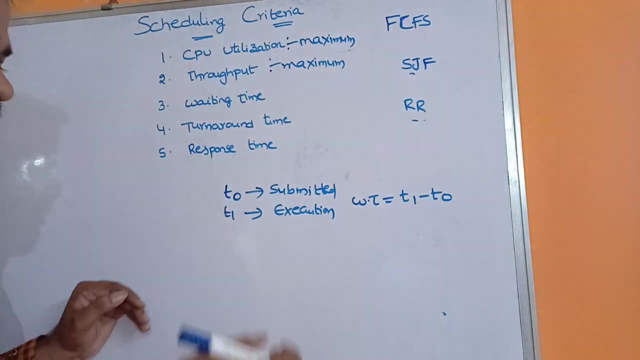 started at time t1.. So t0 is the time at which the process has been submitted in the ready queue, Whereas t1 is the time at which CPU starts its execution. Then we can define waiting as waiting time is equal to t1 minus t0.. So how much time that process is waiting in the 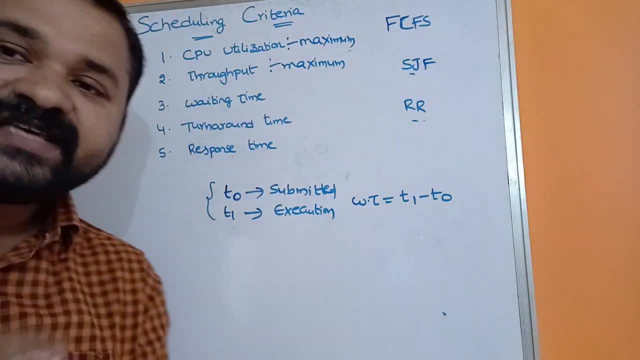 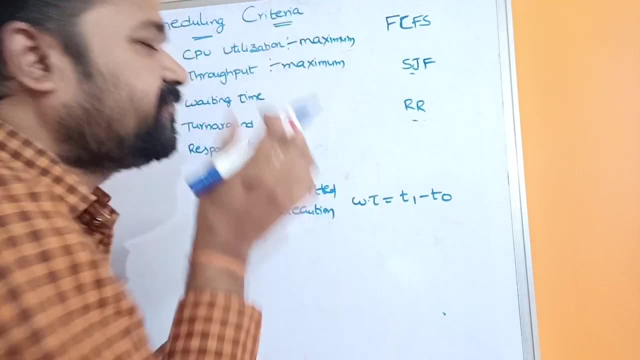 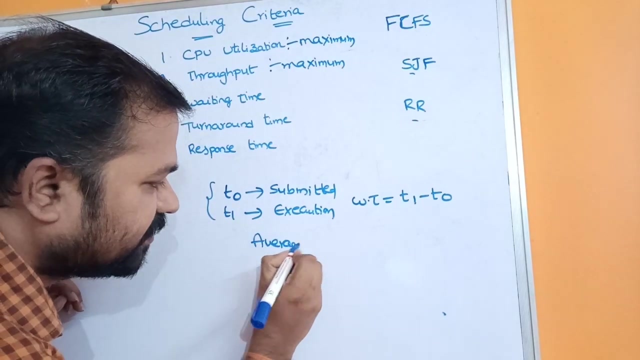 ready queue. So that is nothing but waiting time. So, as a user, what is our target? Waiting time should be minimum. Let us assume that FCFS here if we let we executed five processes. Here we consider average waiting time in order to say whether an algorithm is best. 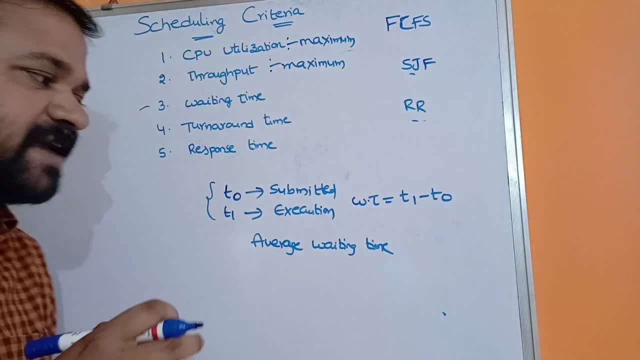 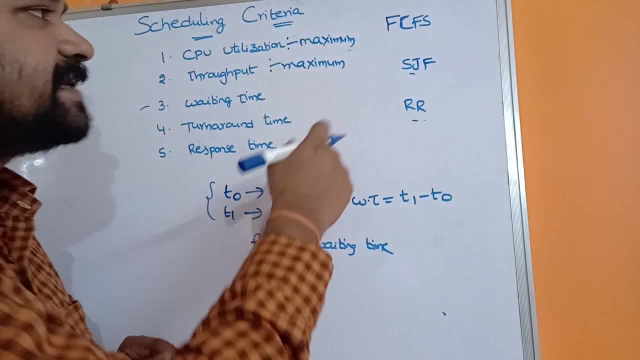 algorithm or not. So if average waiting time is smaller, if average waiting time is minimum, then we can say that that algorithm is the best algorithm. Let us assume that we have taken five processes and we have calculated average waiting time with the help of these. 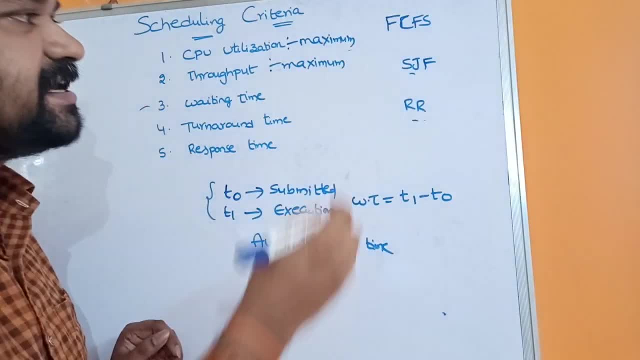 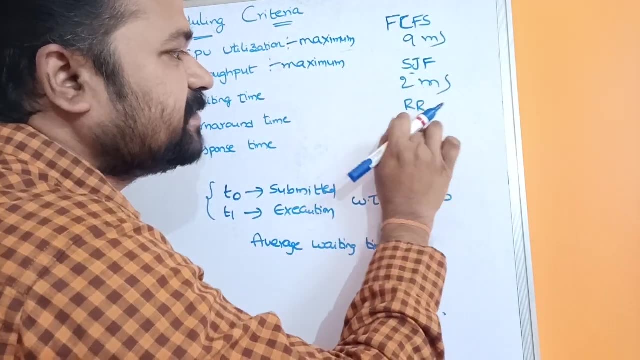 three algorithms. Let us: if we use FCFS, then the average waiting time is some 9 milliseconds, Whereas if we use SAF, then the average waiting time is 2 milliseconds. If we use FCFS, then the average waiting time is 2 milliseconds. If we use FCFS, then the average 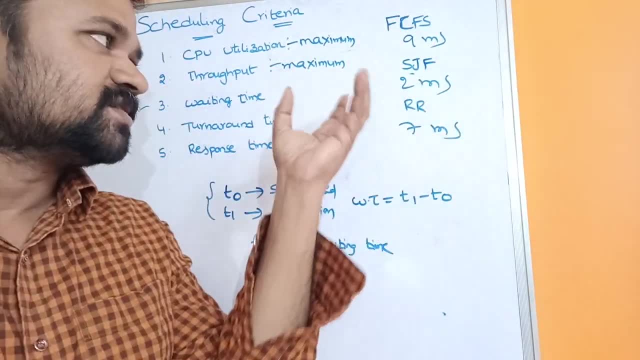 waiting time is 2 milliseconds. If we use FCFS then the average waiting time is 2 milliseconds. Robin let, the average waiting time is 7 milliseconds. so which algorithm has lesser average waiting day? as a F, so we can say that as a F is the best. 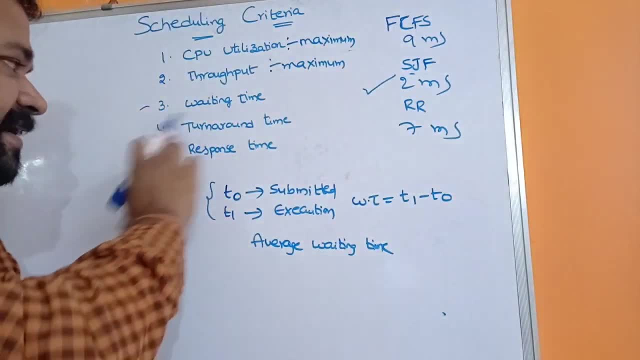 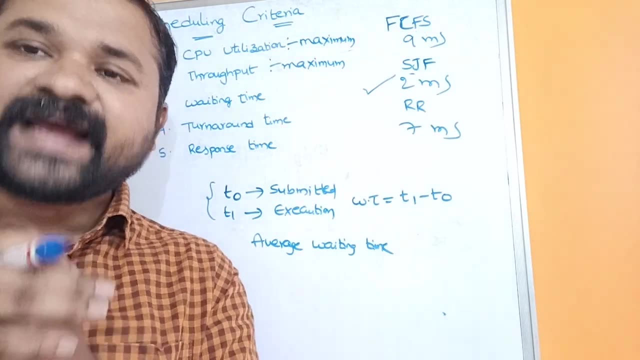 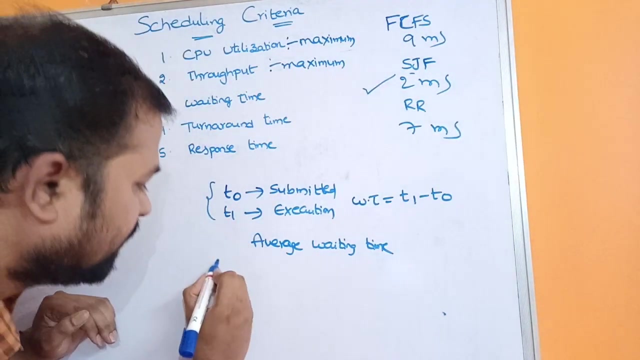 algorithm. so that is about what is waiting time. now let's see about the next one: turn around time, so turn around time. so turn around time means the time duration between the job that is submitted and its completion. let us assume that a process has been submitted, yet time t naught at a time t. 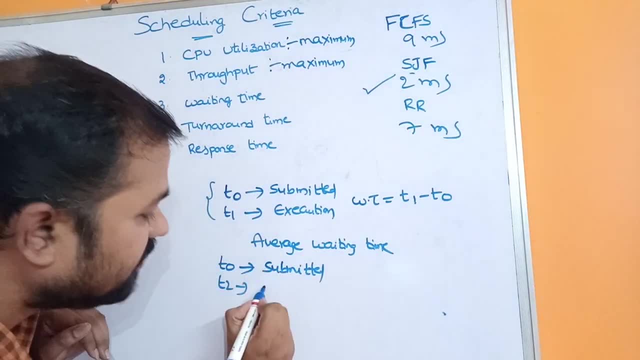 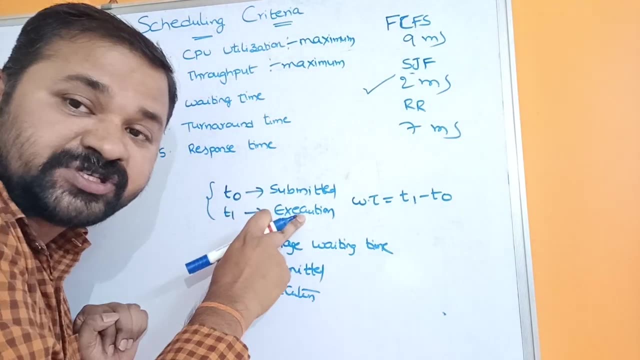 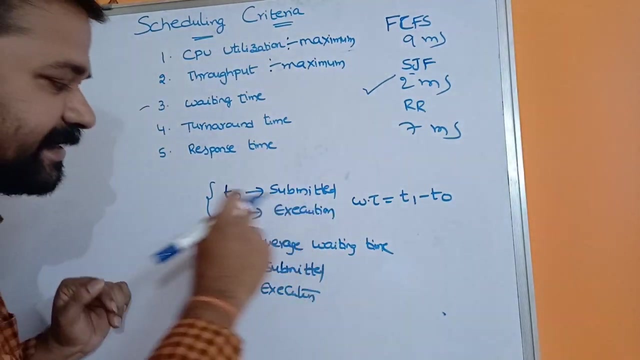 naught where he has. CPU has completed that process execution at time t2. here what is t1? t1 means CPU started that process execution at time t1. okay, so waiting time is equal to that t1 minus t. naught here what is t2? CPU has completed. 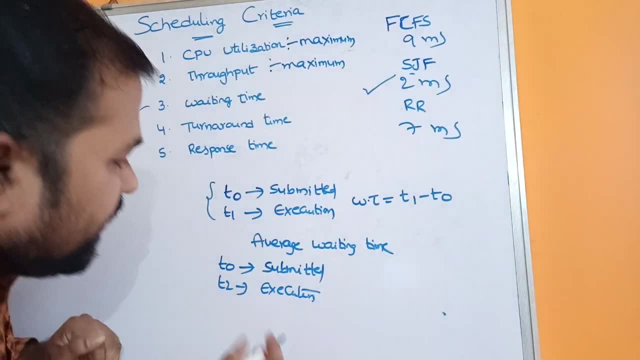 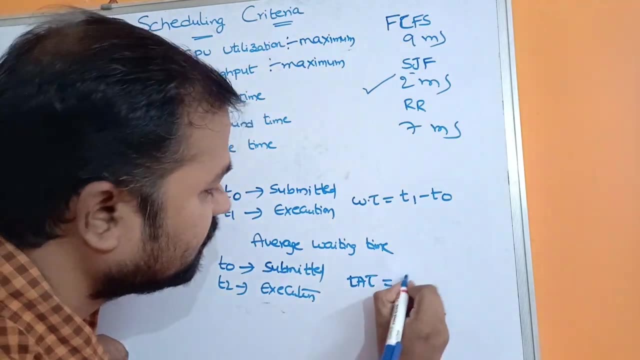 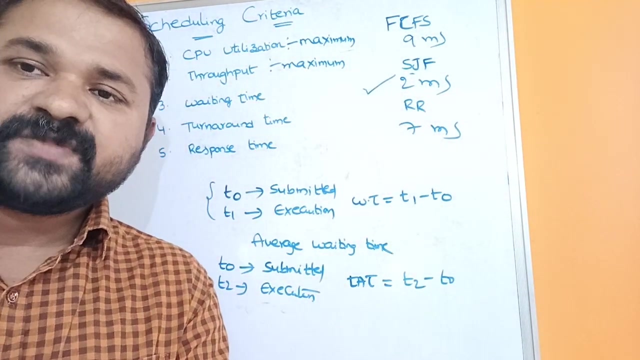 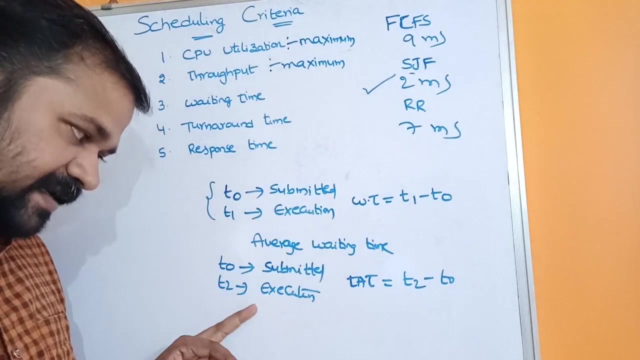 its operations. okay, then we can define average, then we can define: what is the factor here. turnaround time: yes, t2 minus t naught. so what is the definition for turnaround time? turnaround time is the time interval between a process that has been submitted and and the process that completed its execution. so here assumes: 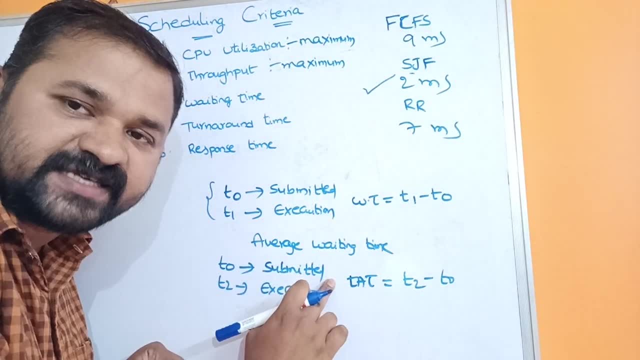 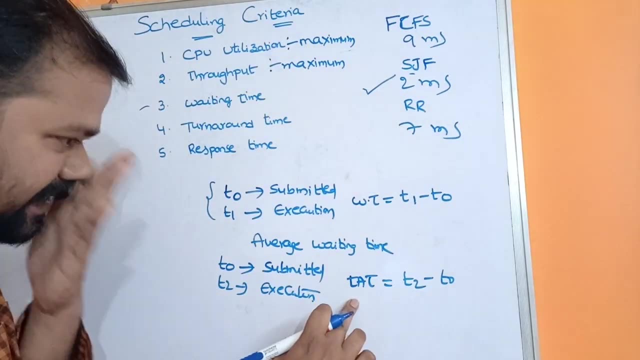 that at a time t naught, we have submitted the process in the ready queue. where, yes, at a time t2 the process has completed its execution. then we can say: turnaround time: yes, t2 minus t naught. so, as i use it, what is our target turnaround time? 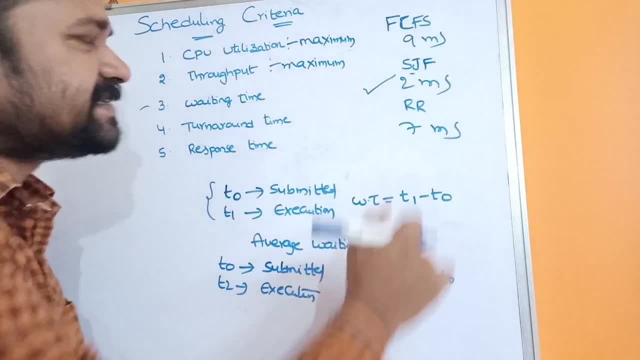 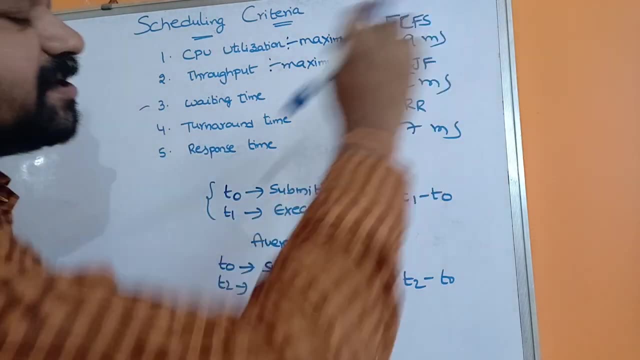 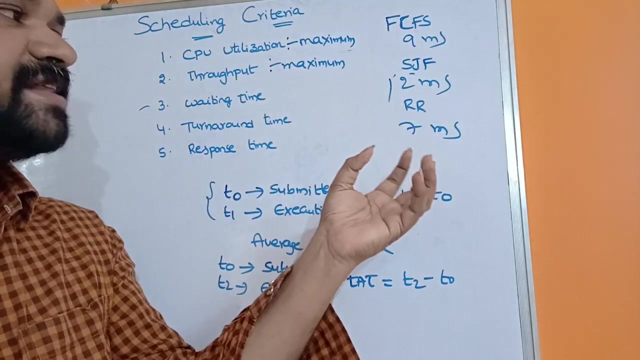 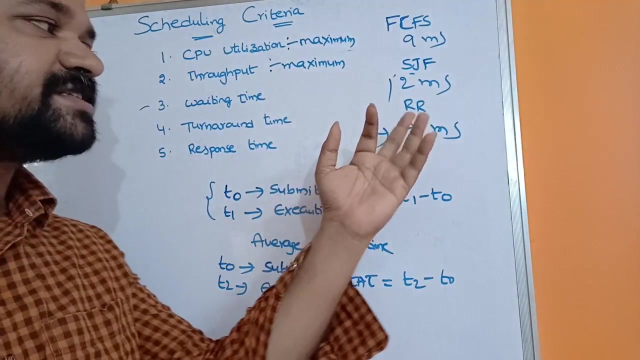 should be minimum. let us take this example and let the turnaround time of FCFS is 9 milliseconds, the turnaround time of sjf is 12 milliseconds. various turnaround time of round robin is 7 milliseconds. So which algorithm is producing lesser average turnaround time? This RR algorithm, round robin algorithm? So we can say that. 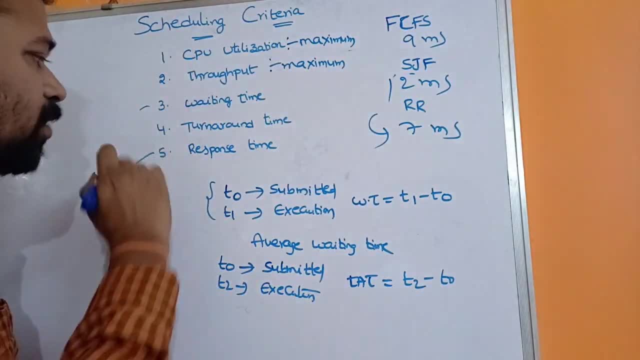 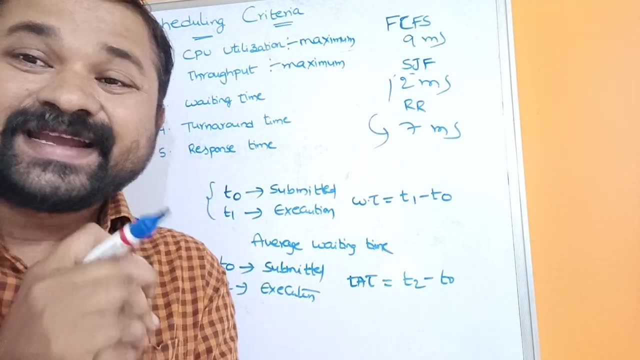 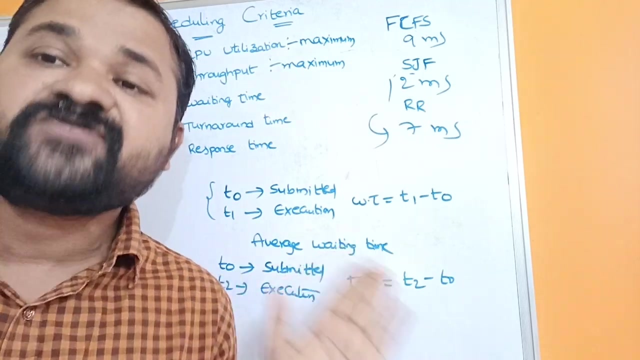 now, round robin algorithm is the best algorithm. Now let us see about response time. So response time means whenever CPU starts executing that process, it has to produce some output. That is called as response Here. response means it is not the final output. So whenever CPU 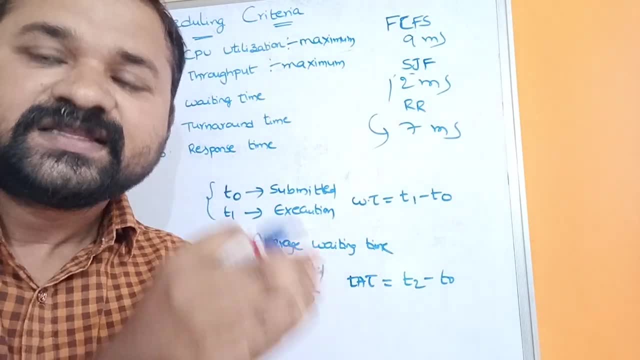 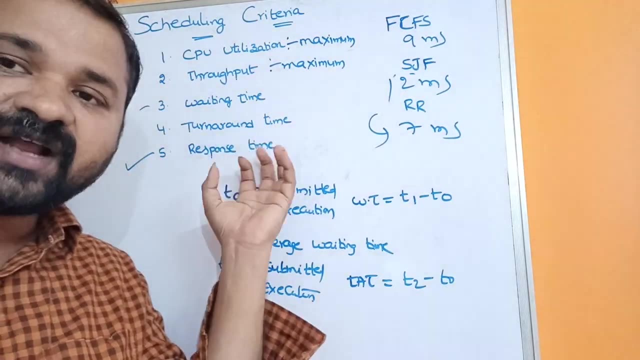 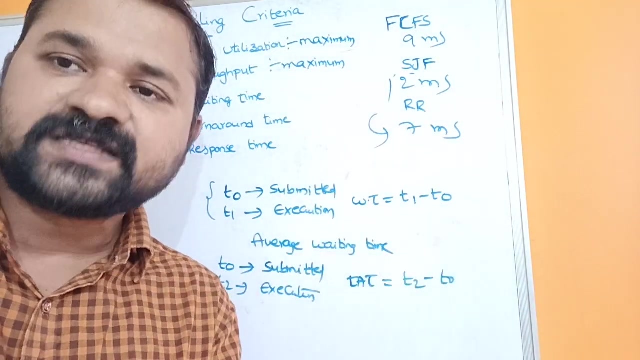 produces a fast output, a fast response, then it is called as response time. Response time is not the final output. So here as a user, our target is response time should be minimum. So whenever the response time is minimum, then we can say that the algorithm is the. 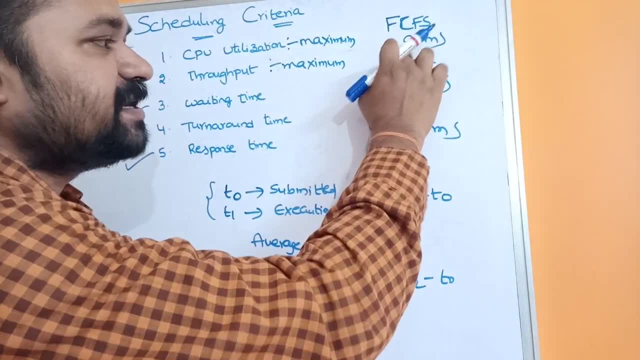 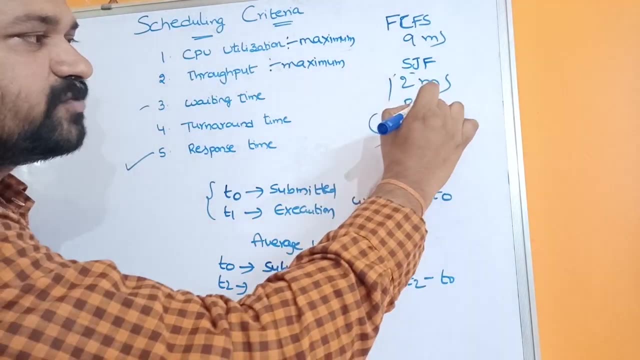 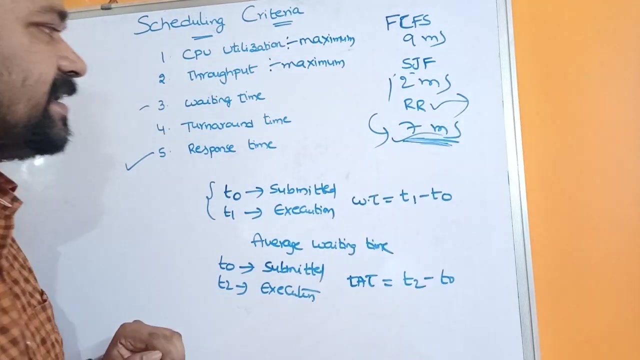 best algorithm. Let the response time for a process here is 9 milliseconds, here 12 milliseconds, here 17.. So what is the minimum value? 7 milliseconds. So if we use a round robin algorithm, then the response time for that process is 7 milliseconds. So we can say that this is the best algorithm. 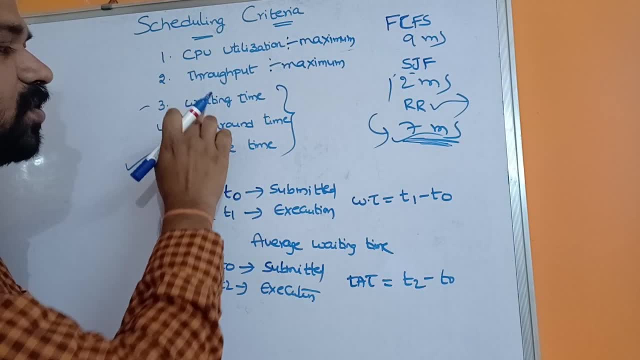 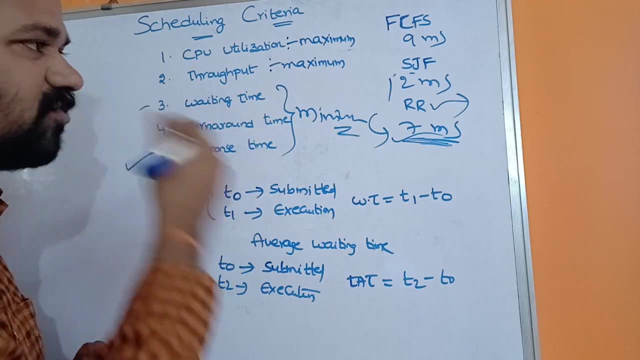 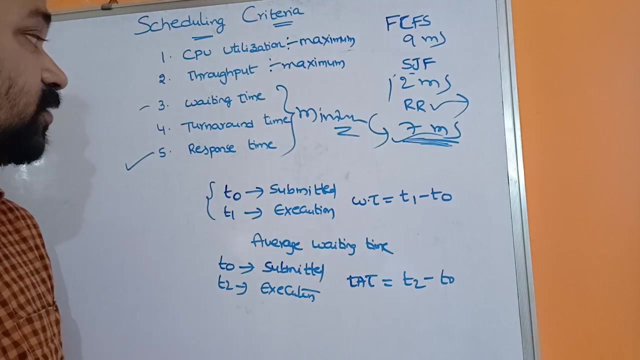 So, as a user, our target is this: waiting time or turnaround time, response time should be minimum. So, in order to calculate the waiting time, what we have to do, We have to calculate average waiting time For turnaround time. we have to calculate average turnaround time.